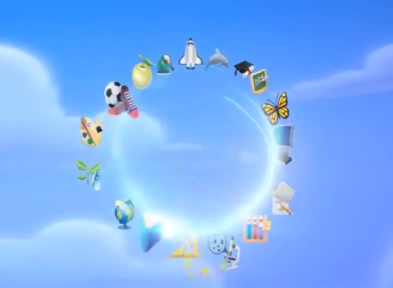 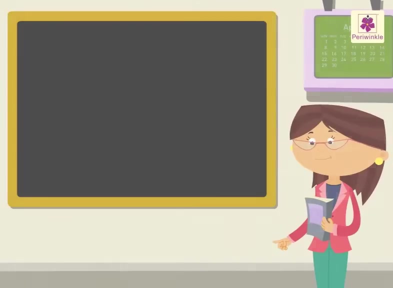 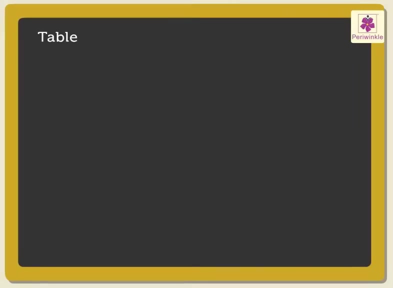 Please add punctuation in the appropriate places. 4 ones are 4.. 5 ones are 5.. 6 ones are 6.. 7 ones are 7.. 8 ones are 8.. 9 ones are 9.. 10 ones are 10.. 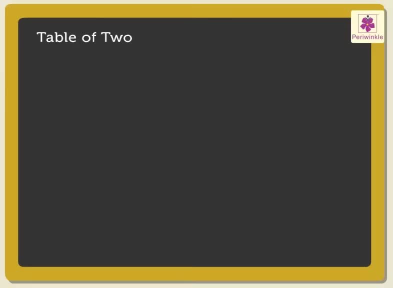 Next is the table. Next is the table of 2.. 1- 2 is 2.. 2- 2s are 4.. 3- 2s are 6.. 4- 2s are 8.. 5- 2s are 10.. 6- 2s are 12.. 7- 2s are 14.. 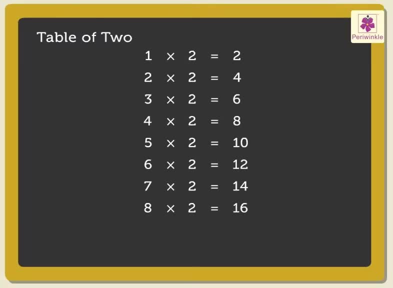 8, 2s are 16.. 9, 2s are 18.. 10, 2s are 20.. Now the table of 3.. 1, 3 is 3.. 2, 3s are 6.. 3, 3s are 9.. 4, 3s are 8.. 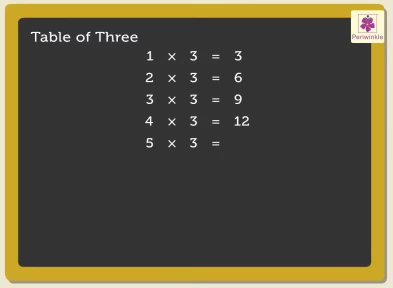 12. 5 3s are 15.. 6 3s are 18.. 7 3s are 21.. 8 3s are 24.. 9 3s are 27.. 10 3s are 30.. 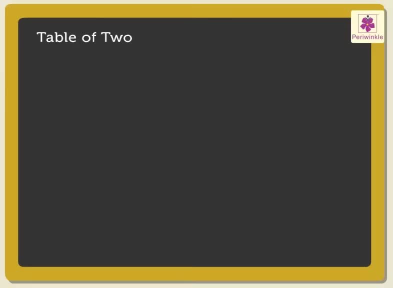 Next is the table. Next is the table of 2.. 1- 2 is 2.. 2- 2s are 4.. 3- 2s are 6.. 4- 2s are 8.. 5- 2s are 10.. 6- 2s are 12.. 7- 2s are 14.. 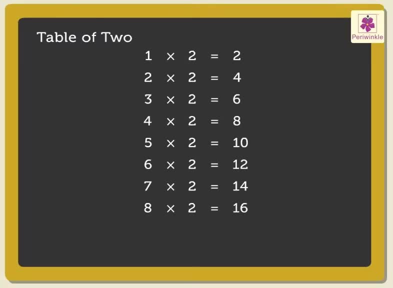 8, 2s are 16.. 9, 2s are 18.. 10, 2s are 20.. Now the table of 3.. 1, 3 is 3.. 2, 3s are 6.. 3, 3s are 9.. 4, 3s are 8.. 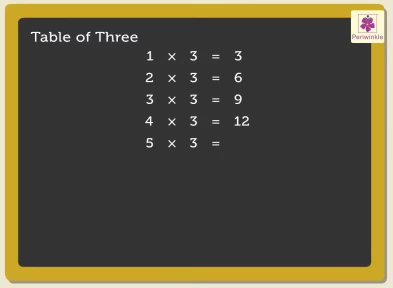 12. 5 3s are 15.. 6 3s are 18.. 7 3s are 21.. 8 3s are 24.. 9 3s are 27.. 10 3s are 30.. 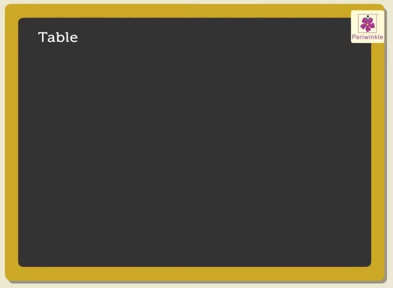 Next is the table of 4.. 1- 4 is 4.. 2- 4s are 8.. 3- 4s are 12.. 4- 4s are 16.. 5- 4s are 20.. 6- 4s are 24.. 7- 4s are 28.. 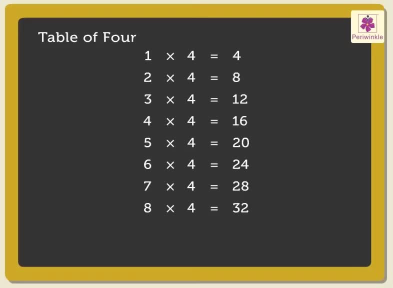 8- 4s are 32.. 9- 4s are 36.. 10- 4s are 40.. Next is the table of 5.. 1- 5 is 5.. 2- 5s are 10.. 3- 5s are 15.. 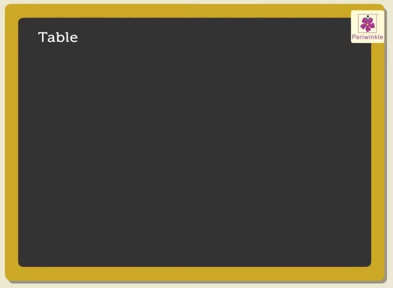 Next is the table of 4.. 1- 4 is 4.. 2- 4s are 8.. 3- 4s are 12.. 4- 4s are 16.. 5- 4s are 20.. 6- 4s are 24.. 7- 4s are 28.. 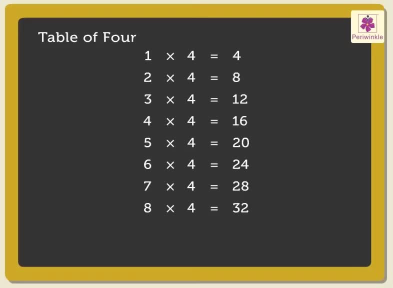 8- 4s are 32.. 9- 4s are 36.. 10- 4s are 40.. Next is the table of 5.. 1- 5 is 5.. 2- 5s are 10.. 3- 5s are 15.. 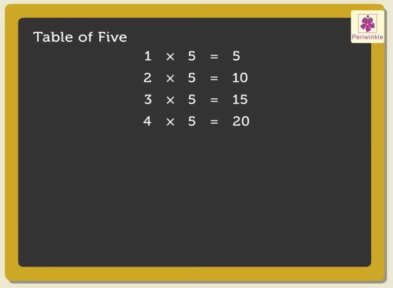 4 5s are 20.. 5 5s are 25.. 6 5s are 30.. 7 5s are 35.. 8 5s are 40.. 9 5s are 45.. 10 5s are 50.. Now the table of 5.. 1 5s are 10.. 10 5s are 40.. 9 5s are 45.. 10 5s are 50.. 10 5s are 50.. 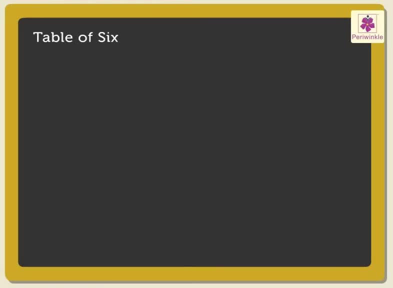 Now the table of 6.. 1- 6 is 6.. 2- 6s are 12.. 3- 6s are 18.. 4- 6s are 24.. 5- 6s are 30.. 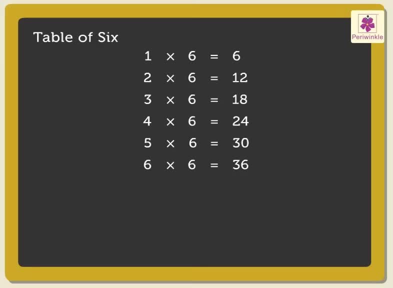 6, 6s are 36.. 6, 6s are 36.. 6, 6s are 36.. Sixes are forty-two. Eight sixes are forty-eight. Nine sixes are fifty-four. Ten sixes are sixty. 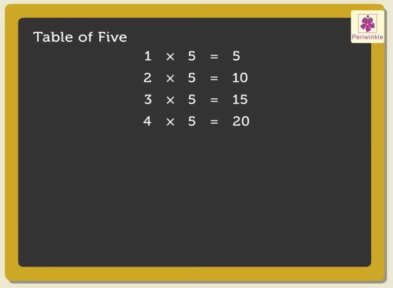 4 5s are 20.. 5 5s are 25.. 6 5s are 30.. 7 5s are 35.. 8 5s are 40.. 9 5s are 45.. 10 5s are 50.. Now the table of 5.. 1 5s are 10.. 10 5s are 40.. 9 5s are 45.. 10 5s are 50.. 10 5s are 50.. 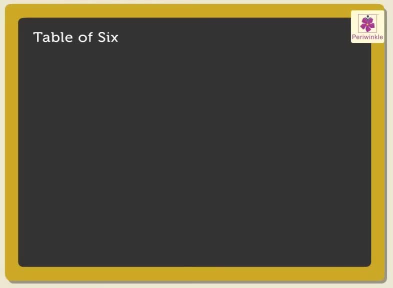 Now the table of 6.. 1- 6 is 6.. 2- 6s are 12.. 3- 6s are 18.. 4- 6s are 24.. 5- 6s are 30.. 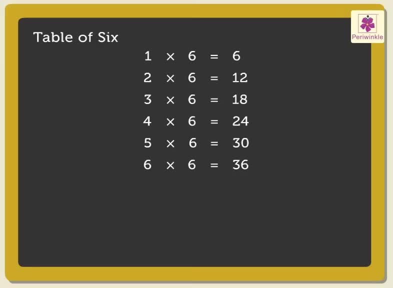 6 6s are 36.. Seven sixes are forty-two. Eight sixes are forty-eight. Nine sixes are fifty-four. Ten sixes are sixty. Next is the table of seven. One seven is seven. Two sevens are fourteen. 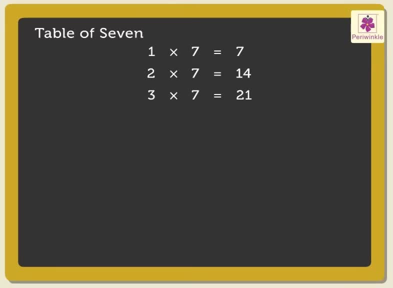 Three sevens are twenty-one. Four sevens are twenty-eight. Five sevens are thirty-five. Six sevens are forty-two. Seven sevens are forty-nine. Eight sevens are fifty-six. Nine sevens are sixty-three. Ten sevens are seventy. 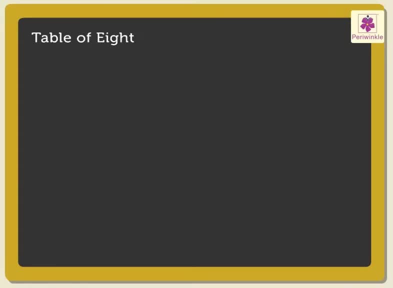 Now let us revise the table of eight. One eight is eight. Two eights are sixteen. Three eights are twenty-four. Four eights are thirty-two. Five eights are forty. Six eights are twenty-eight. Seven eights are forty-eight. 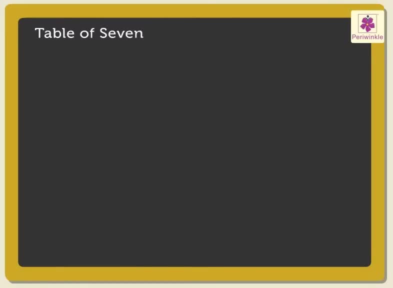 Next is the table of seven. One seven is seven. Two sevens are fourteen. Three sevens are twenty-one. Four sevens are twenty-eight. Five sevens are thirty-five. Six sevens are forty-two. Seven sevens are forty-nine. 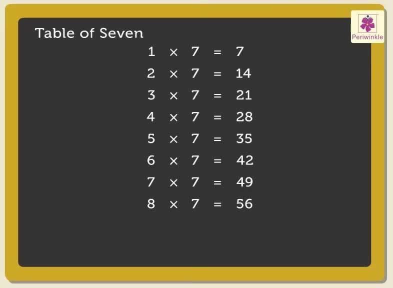 Eight sevens are fifty-six. Nine sevens are sixty-three. Ten sevens are forty-nine. Seven sevens are seventy. Now let us revise the table of eight. One eight is eight. Two eights are sixteen. Three eights are twenty-four. 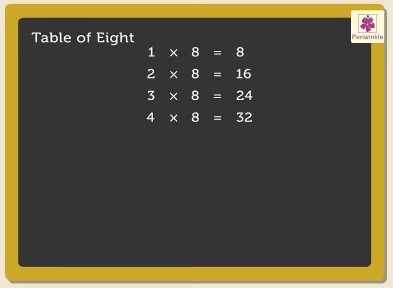 Four eights are thirty-two. Five eights are forty. Six eights are forty. Seven eights are fifty-six. Eight eights are sixty-four. Nine eights are seventy-two. Ten eights are eighty. Next is the table of nine. 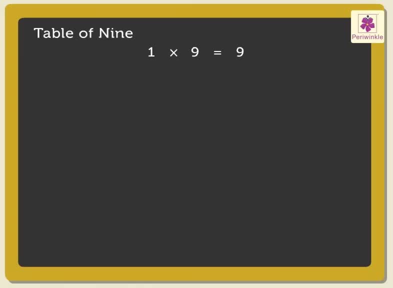 One nine is nine. Two nines are eighteen. Three nines are sixty. Nines are twenty-seven. Four nines are thirty-six. Five nines are forty-five. Six nines are fifty-four. Seven nines are sixty-three. 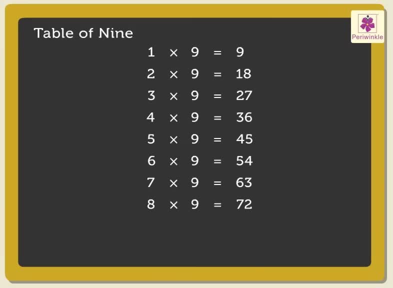 Eight, nines are seventy-two. Nine, nines are eighty-one. Ten nines are ninety. Lastly, the table of ten. One ten is ten. Two tens are twenty. Three tens are thirty. Four tens are forty. Five tens are fifty.